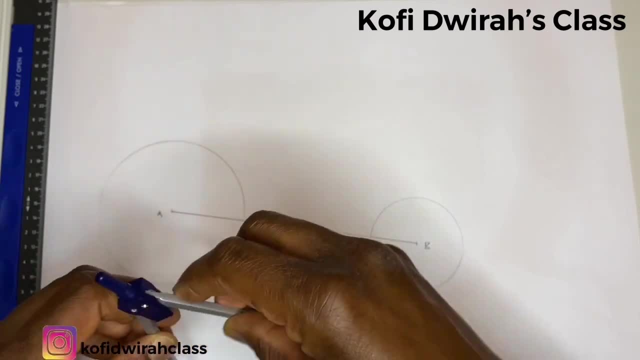 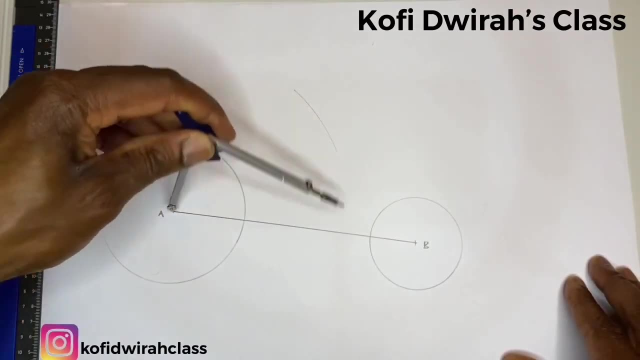 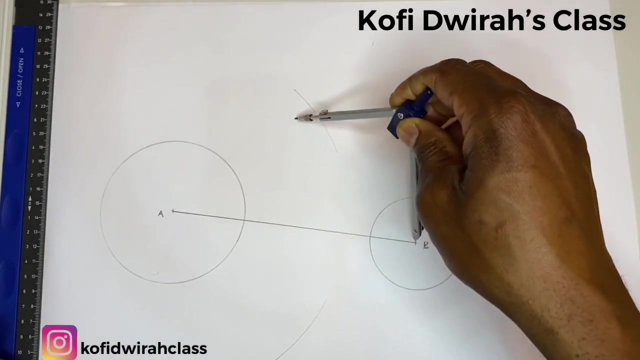 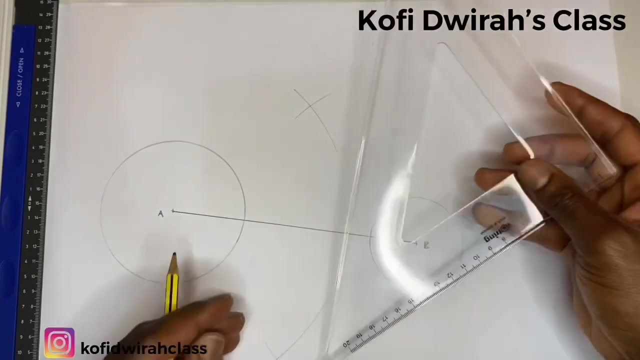 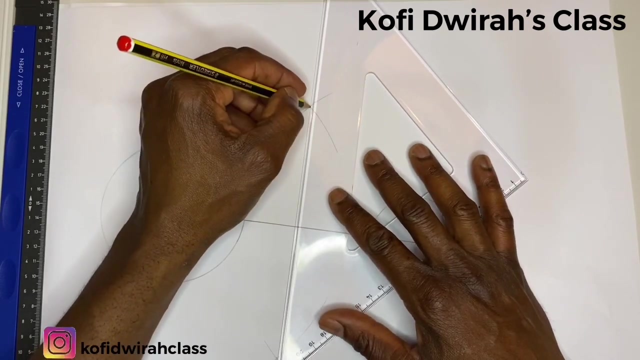 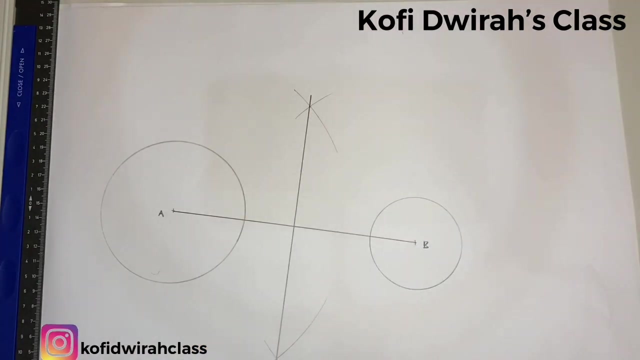 That's it. This is the white line And the horizontal line, Then fictional voice, Then to the left. That's it. and with your compass, at point A you draw an arc, at point B, draw another arc. so we have here, and you draw a straight line. good, then they have a, B. there we have point C. 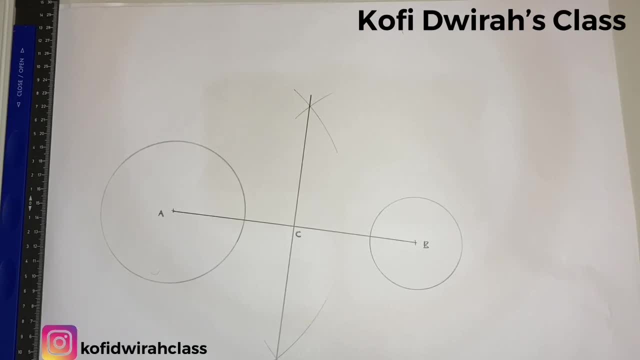 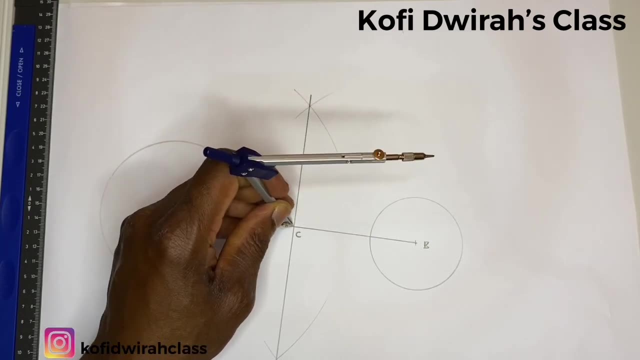 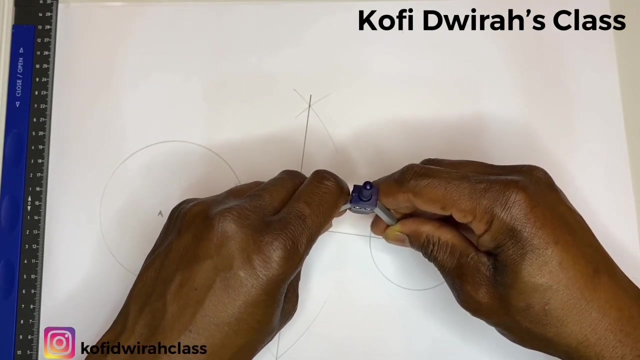 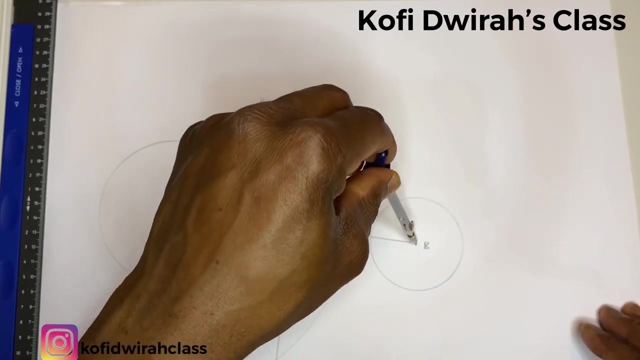 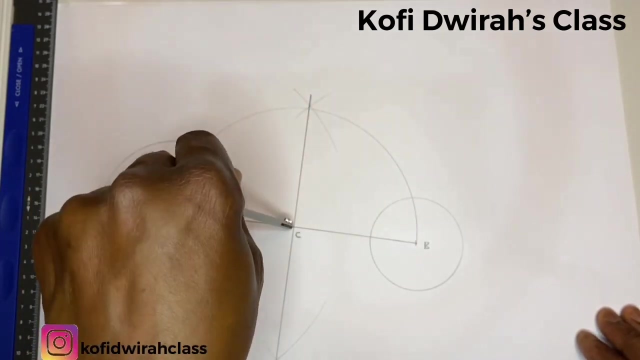 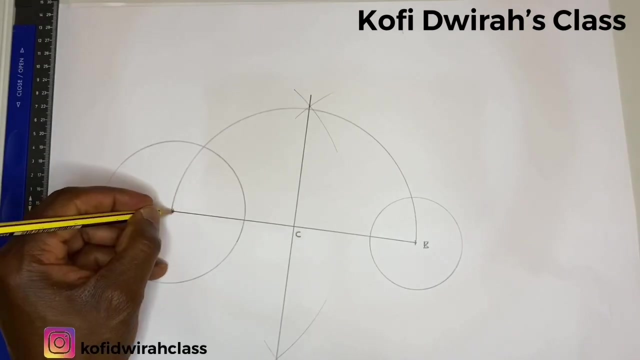 then, with your compass, at point C, you draw a semicircle at point C, at point C, and from you draw a semicircle and it's A- B. you draw a semicircle and it's A- B. good, so this point, we have point A and point B. 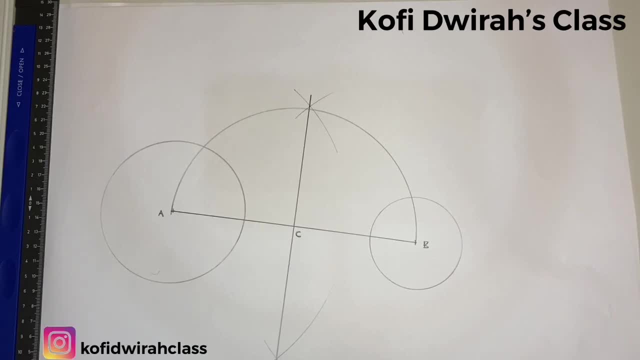 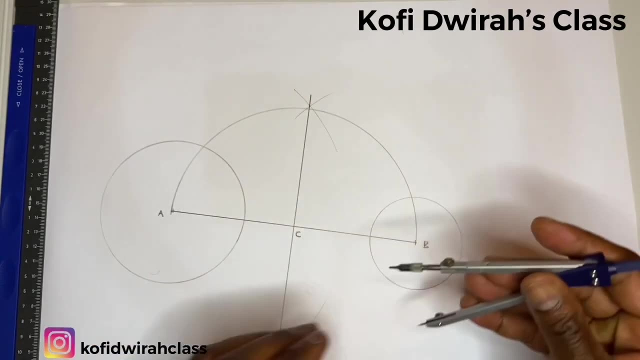 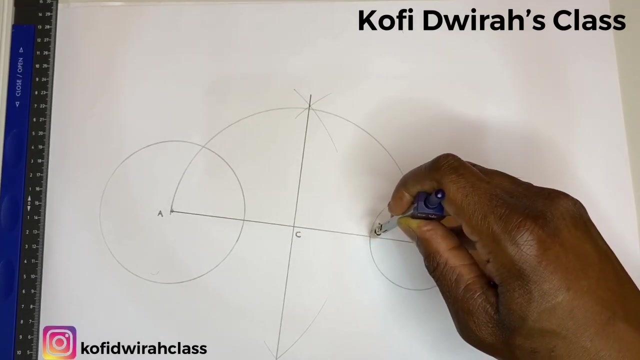 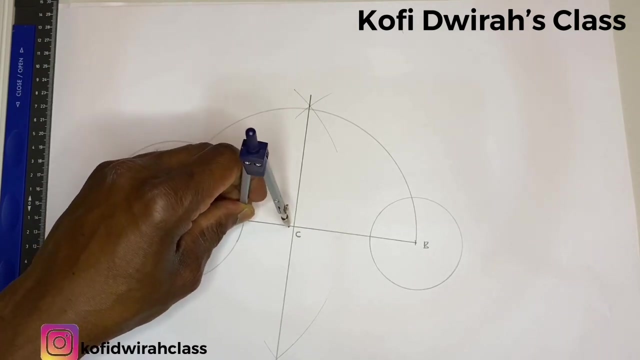 then we have our semicircle. then you measure the radius of the smaller circle. the radius of the smaller circle, you measure it like this, then you add it to the bigger circle, then you add it to the bigger circle. so it's here. so we have this point to be. 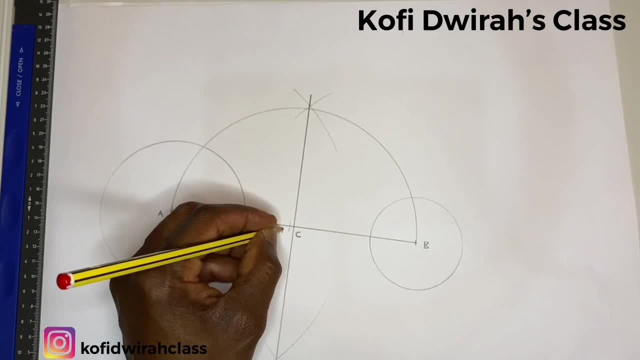 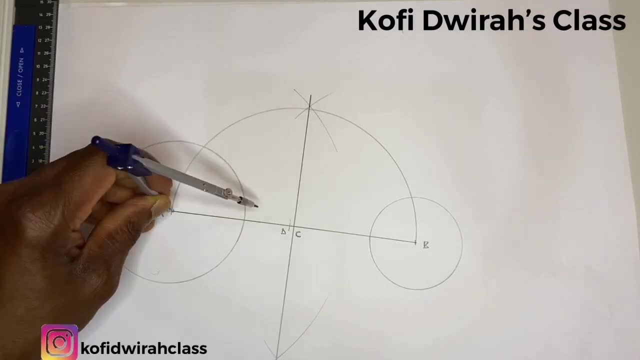 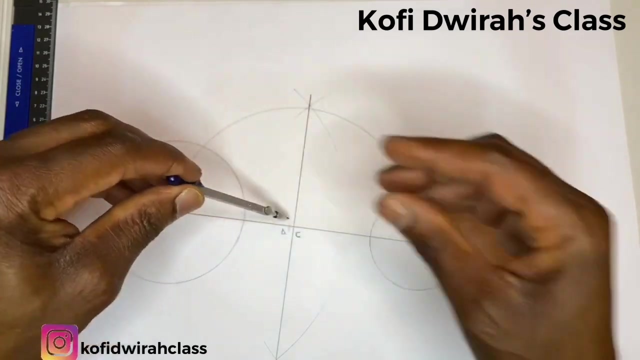 D, then from A open your compass to D, then you draw a semicircle at point A, then you draw a semicircle at point B, then you draw a semicircle at point B, then you draw a semicircle at point C and draw an arc. 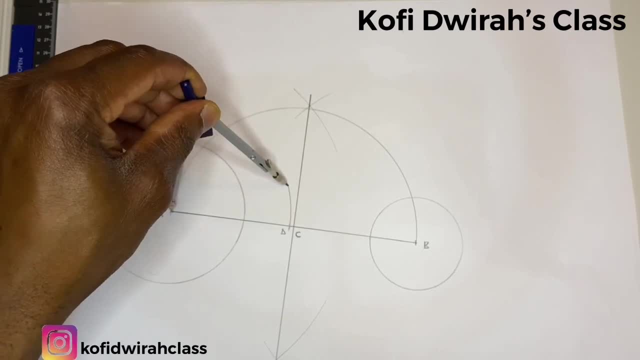 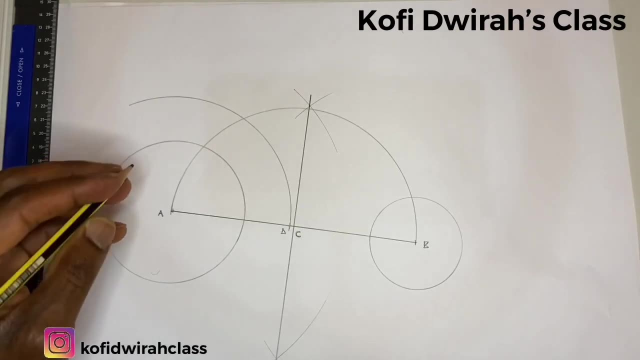 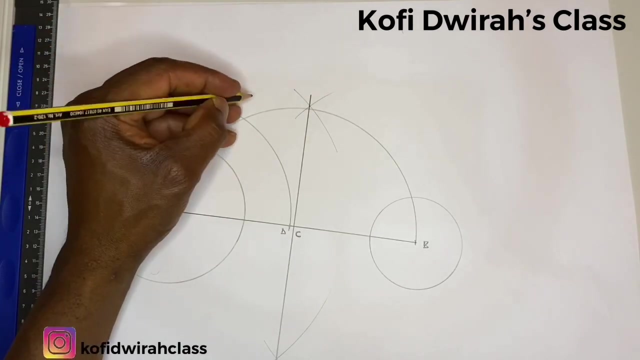 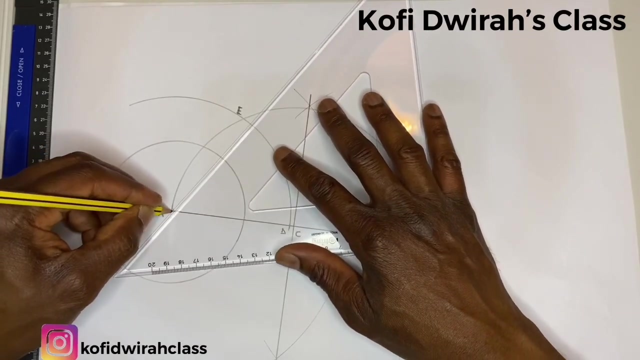 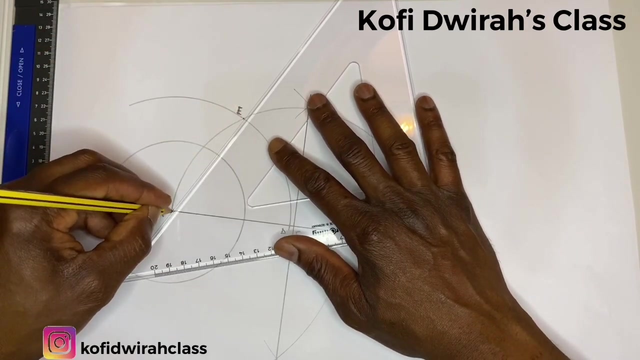 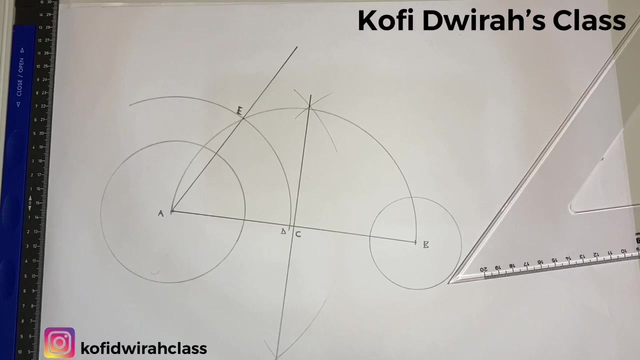 and draw an arc, draw a semicircle at point A, like this. then you draw a straight line like this. then you draw a straight line and make this point here, from A to this point, from A to this point here, from here to here, draw a straight line. good, then we have this. this line is a normal. 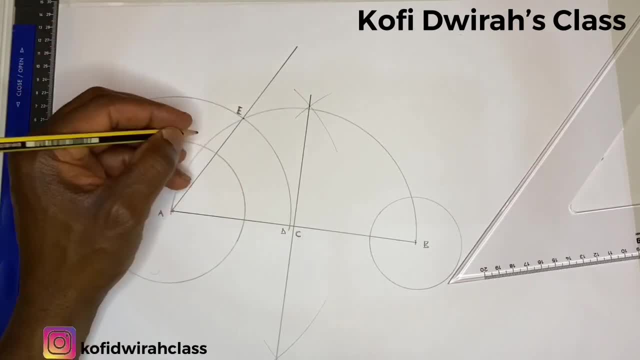 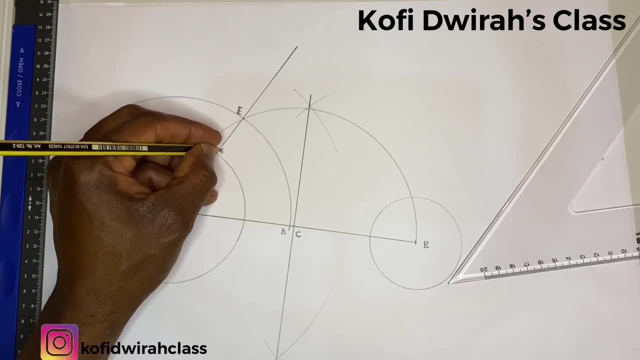 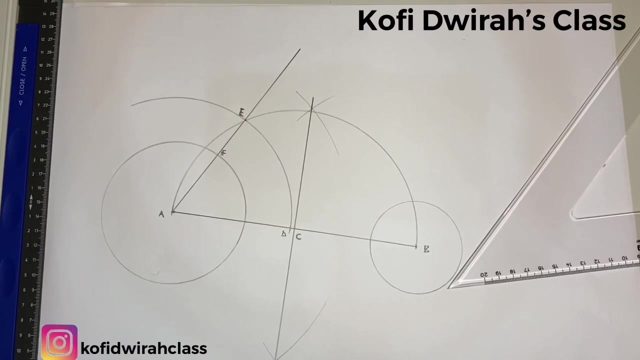 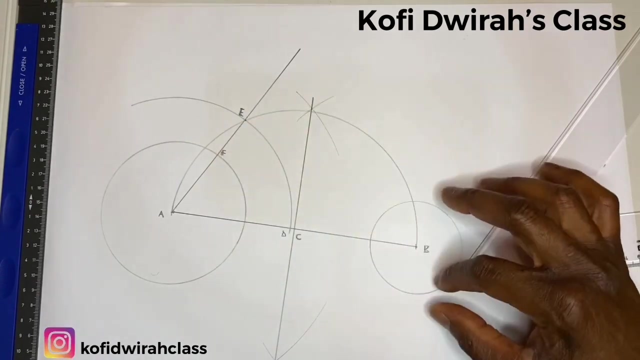 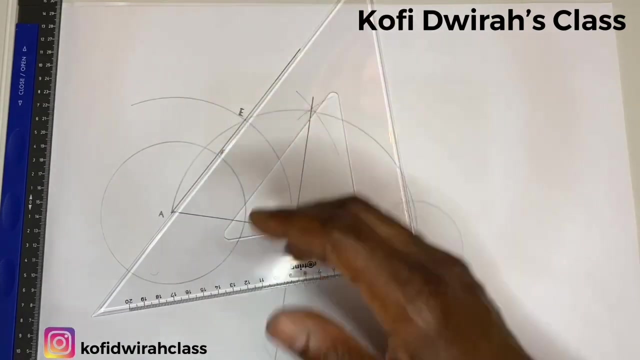 this line is a normal, so we have this point to be point F. yeah, it's the point F. then, with your set squares, you transfer the normal from the bigger circle to the smaller circle. you transfer the normal. this is the normal, so you transfer it and you use the same method. the method. 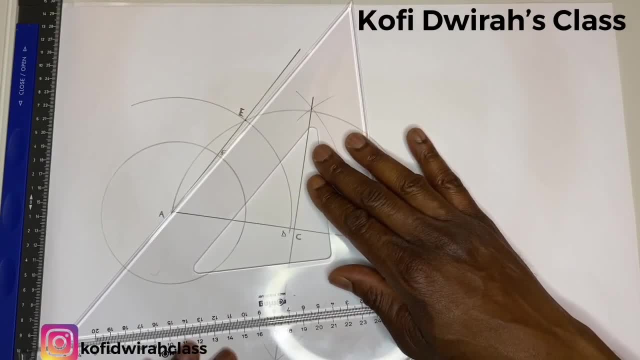 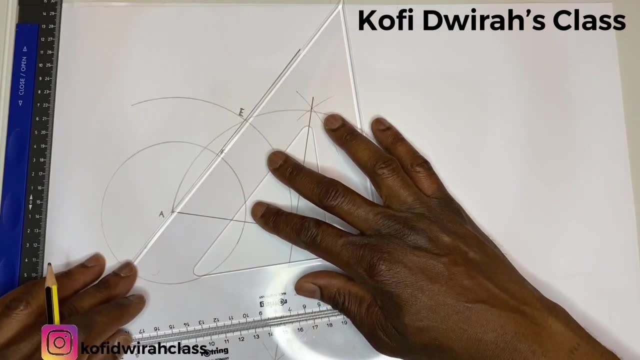 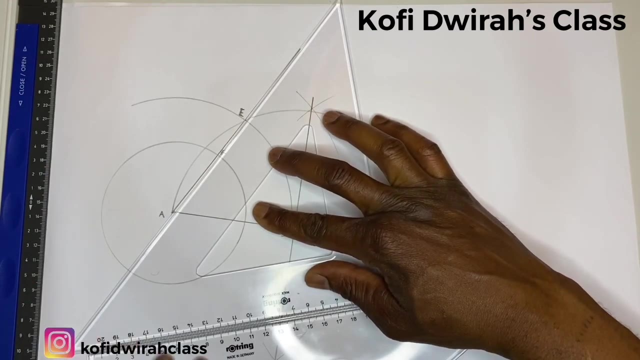 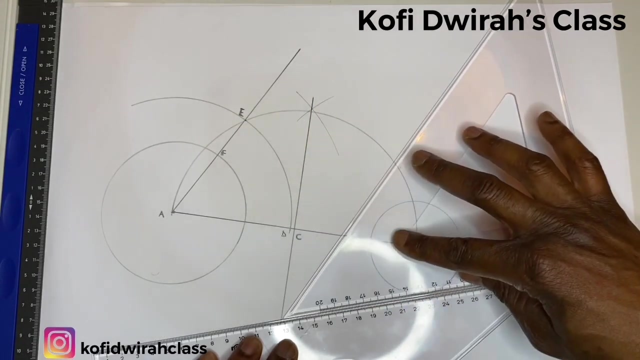 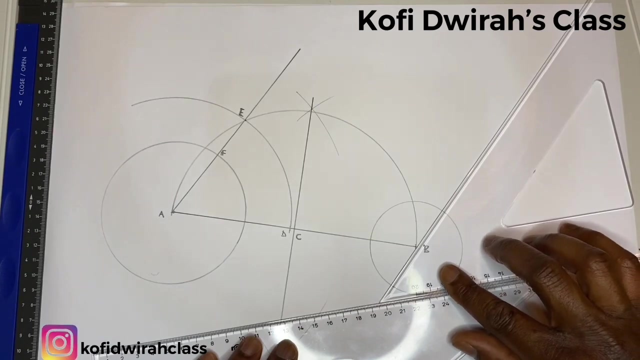 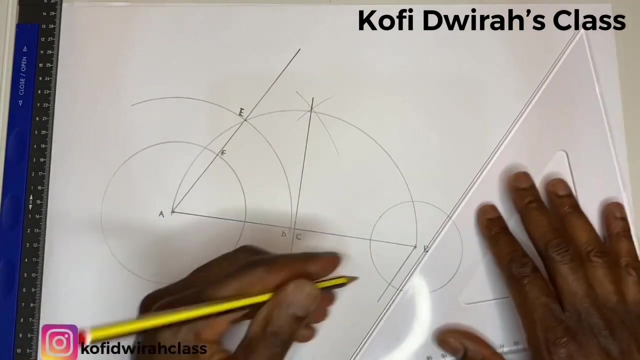 for transferring lines or when you are dividing lines to equal parts. the same method. so you first put a set square like this, then you put this underneath like this, then just move the set square, load the upper one slowly, slowly to B, then you draw your line after 단h getting it. 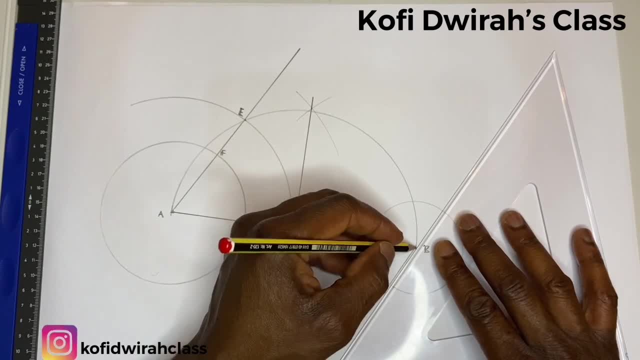 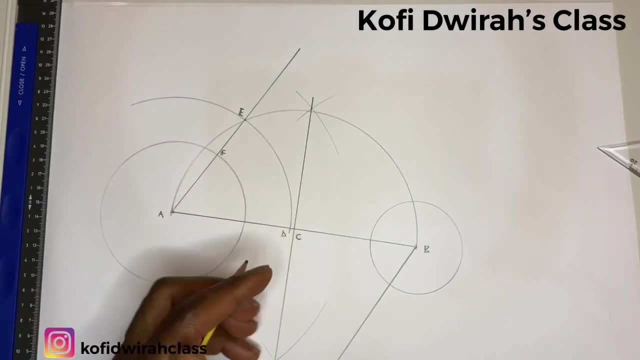 you can just extend it a bit. good, so we have 2 normal. this is normal, that's the minimum. 1, 1.6.3 is all right. The line from the center through the circumference. This is the normal and we have another one here. So we have this point to be point G Right here, like this. Then you draw a straight line, The tangent, From F to G.